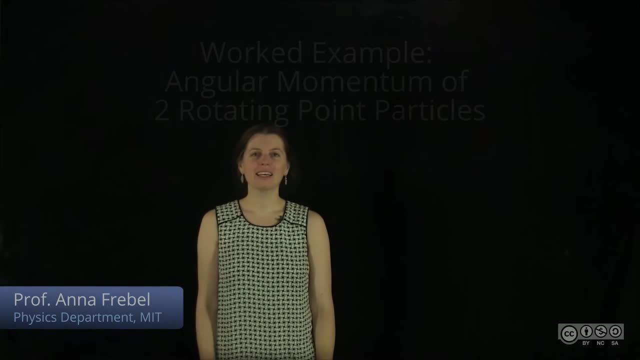 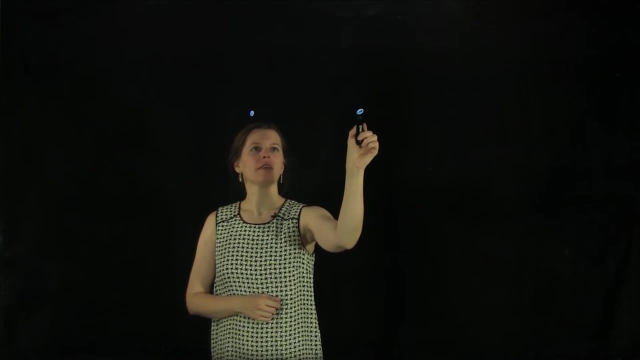 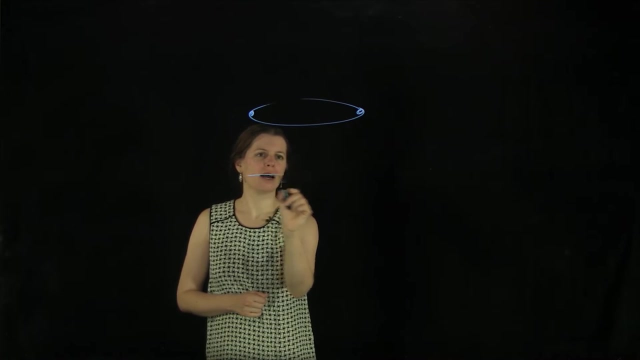 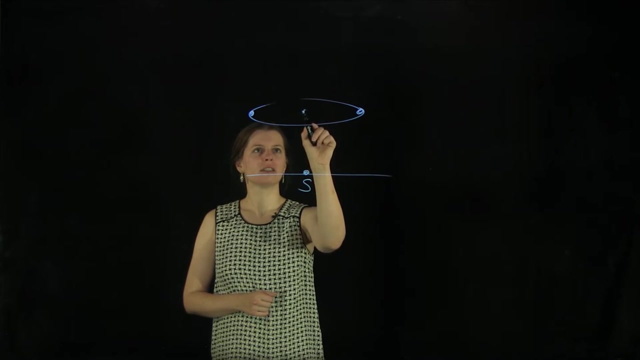 Let's look at the angular momentum of two particles, one sitting here and one over there, And they are circling each other And we want to determine the angular momentum of a point on the ground right here underneath. That's our point S And here is the center, so the 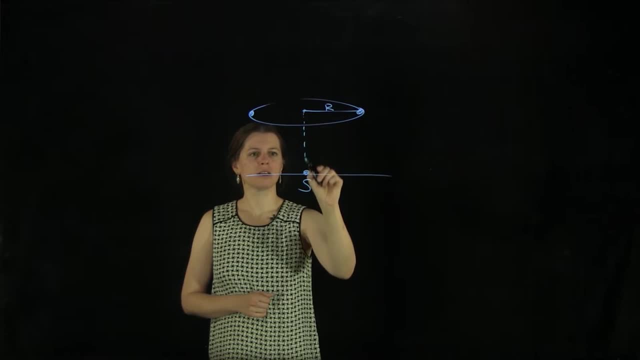 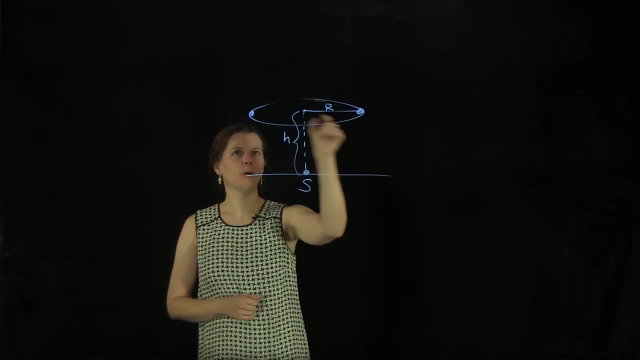 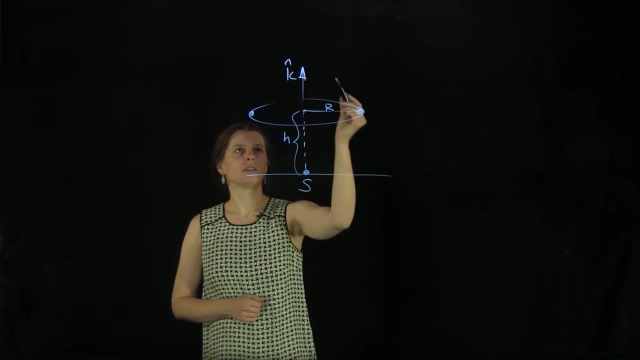 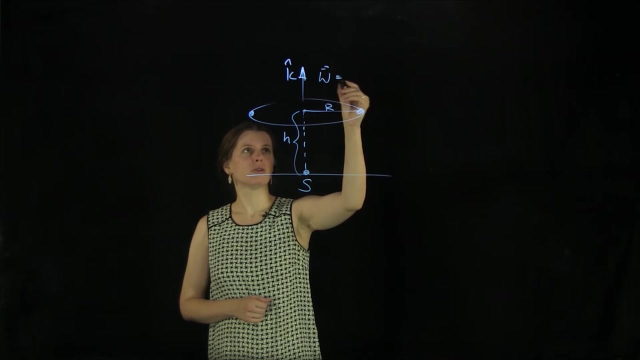 circle has a radius r And here we have a height h. And let's have the particles go counterclockwise, because then we can define our k-head vector to go up, And if these particles are going this way, then omega is also going to be going in the k-head direction in the 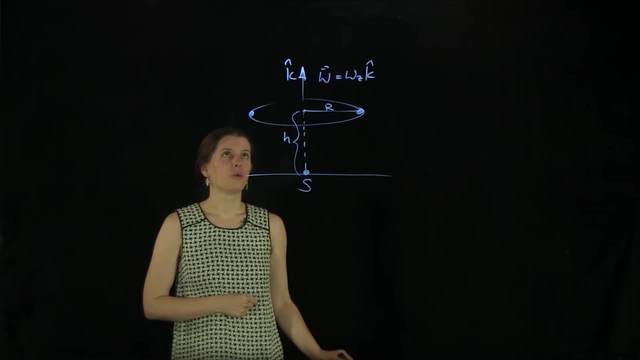 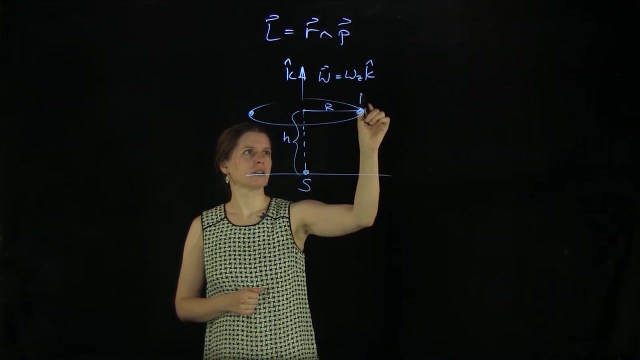 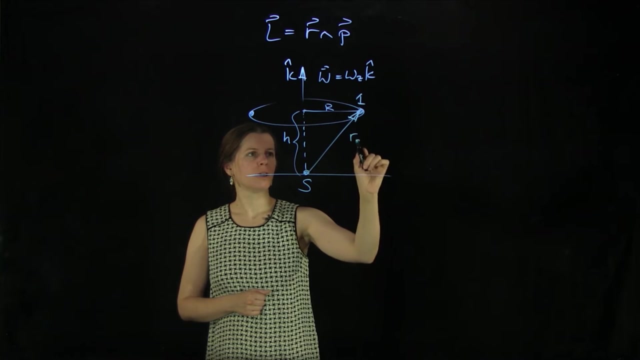 positive direction. So we know that l equals r, cross p. So we need to determine where is r and what's going on with p. So our r vector goes here, from point S to our first particle, rs1.. And here is number 2.. 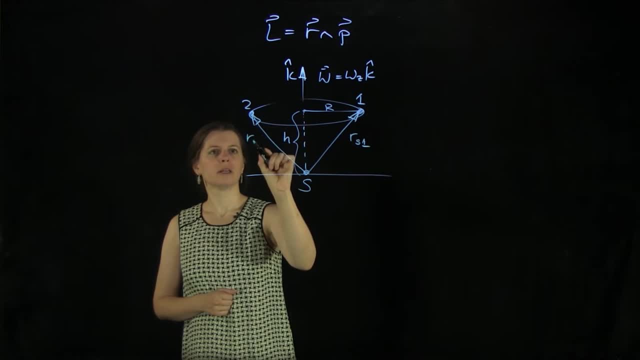 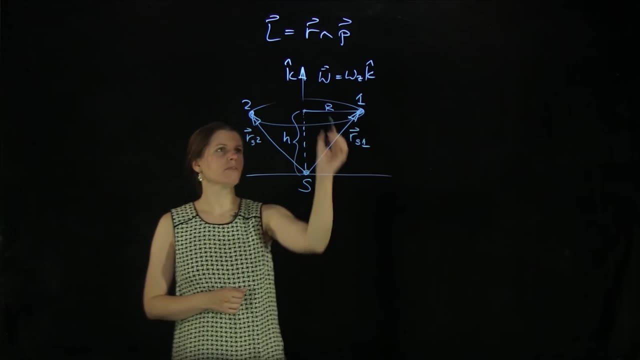 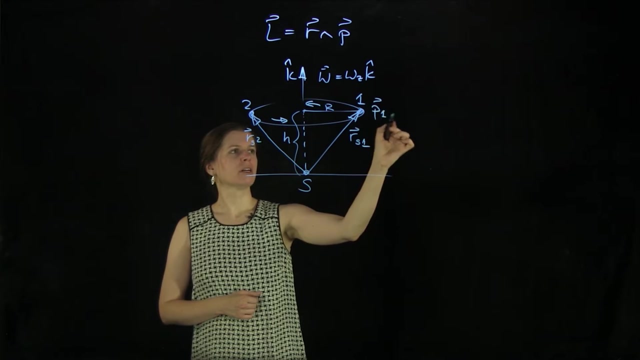 And we have rs1.. And we have rs2 sitting over here And p the momentum of the particles. well, if these guys are going in the counterclockwise direction, then the momentum of particle 1 is going to go into the board following the. 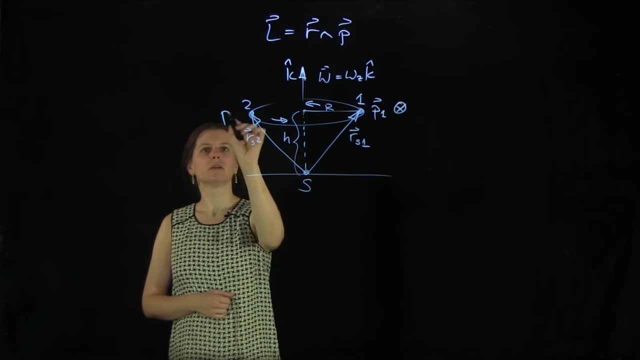 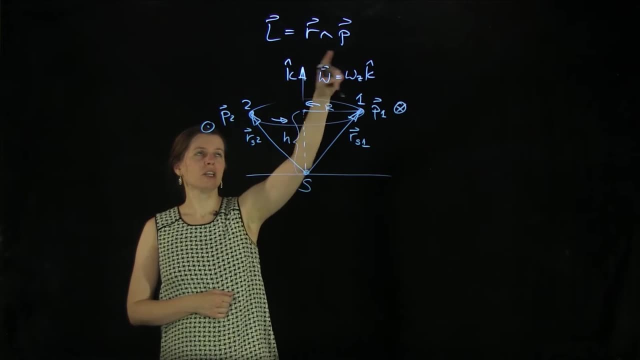 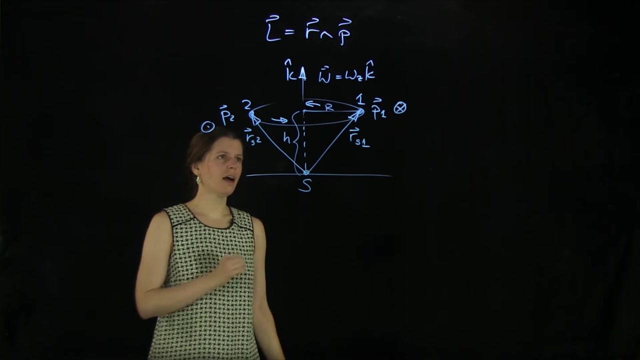 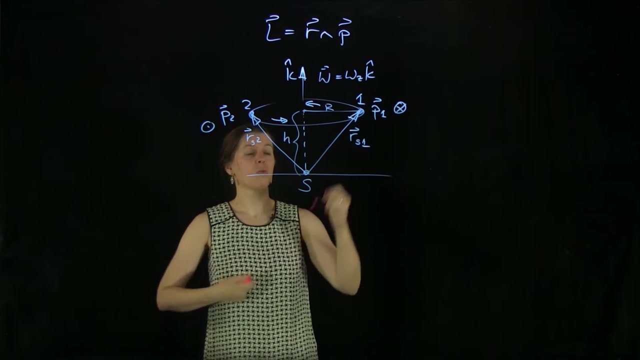 direction of the motion, And here p2 is going to come out of the board. If we consider this equation- And here we can already graphically determine what the answer is actually going to be- And so we do r cross p, So r cross p, which means l, l1, ls1 is going to point in this: 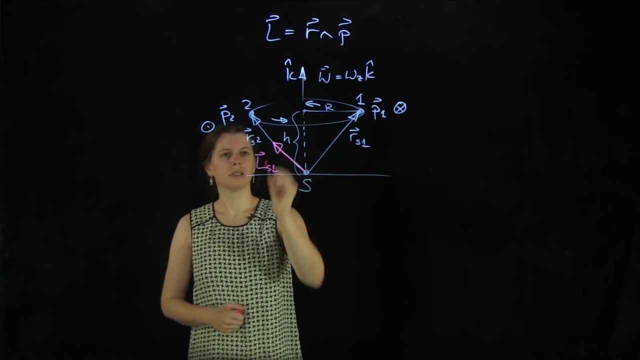 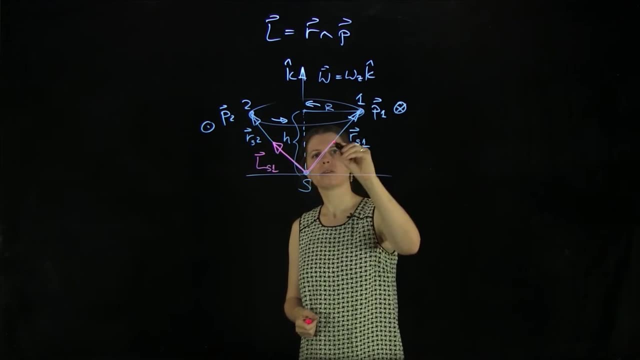 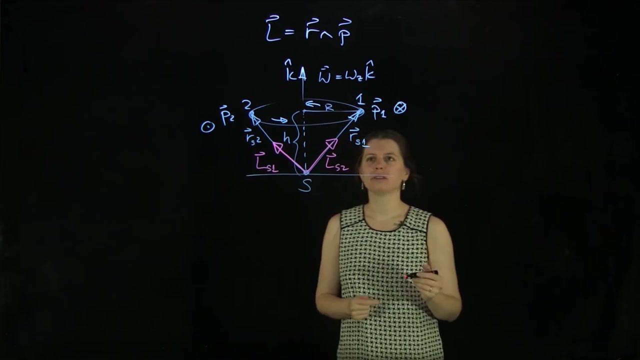 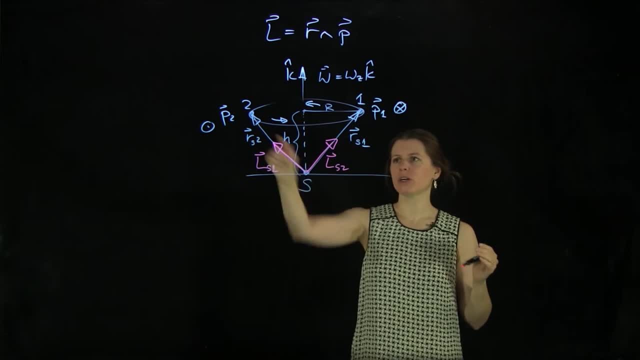 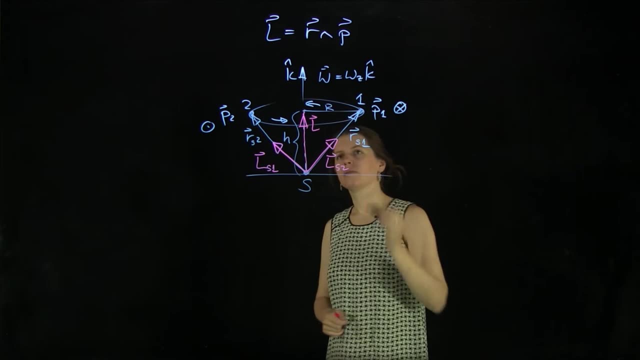 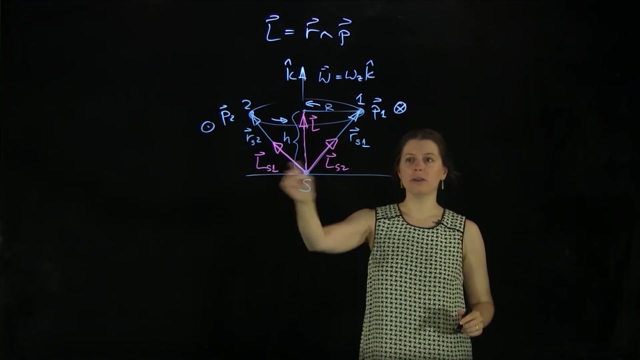 and we do want the total angular momentum of the system of both particles, so we have to add them. we'll get here our l of this system. So in order to calculate that, we need to calculate first the ls1 and then the ls2.. 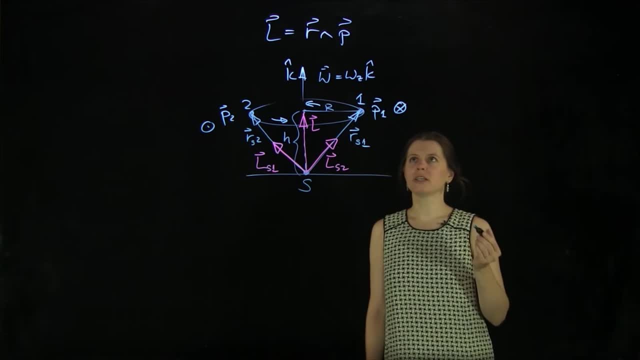 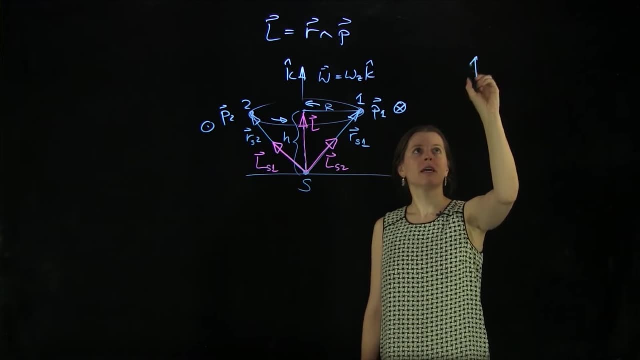 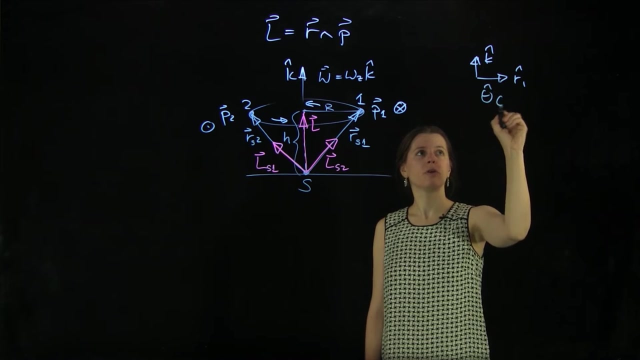 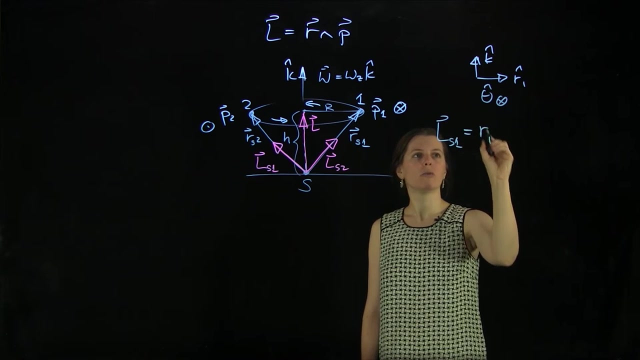 And then we need to add them. The crucial point here is to be careful with the coordinate system, For the first particle, k is going up and r is going outward and theta hat is going into the board. Then we can write up: ls1 equals r1 or s1 cross p1. 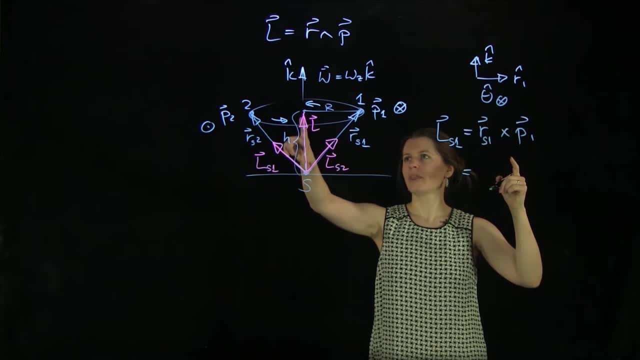 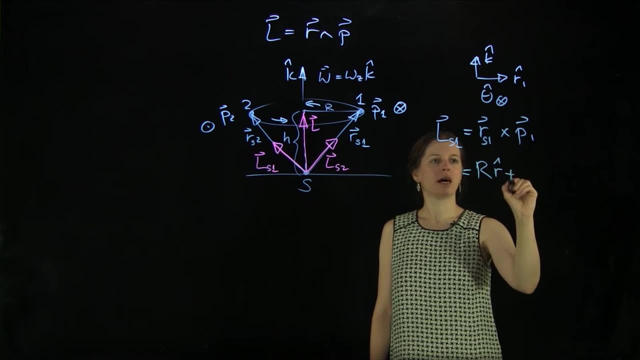 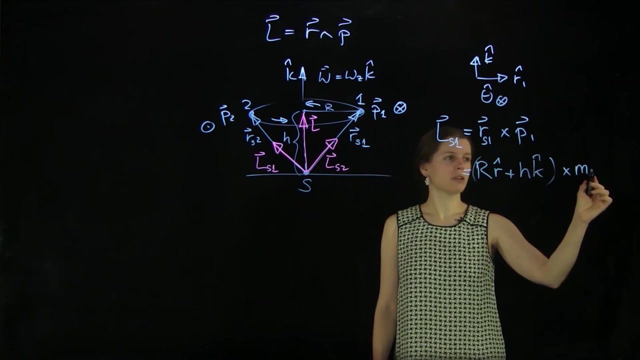 And we can express this vector here with h and with r. So we have r in the r hat direction plus h in the k hat direction, cross p, And p is the mass of the particle times, the angular velocity, the component, That is, r, omega z. 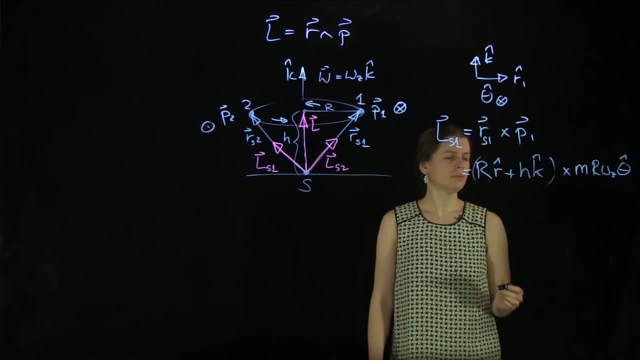 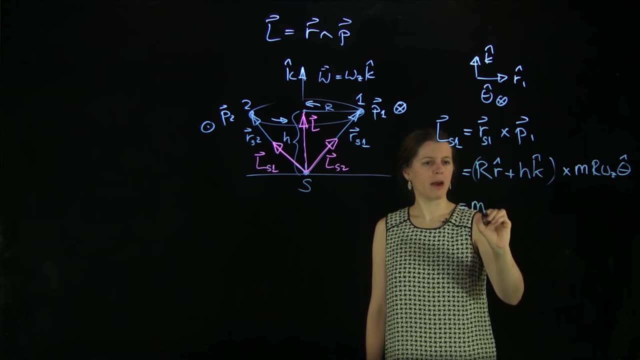 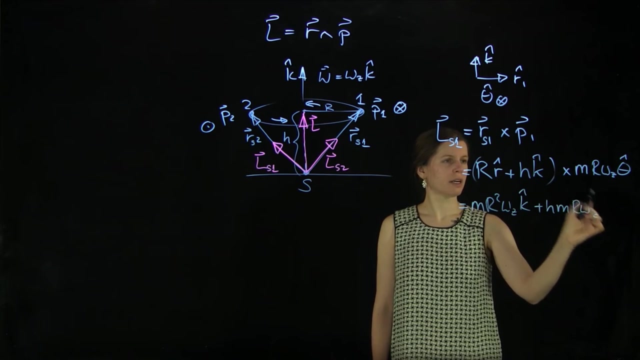 And that goes in the theta direction. So we need to solve this cross This product. here we're going to have m r squared omega z, And then we have r hat cross theta hat, That's k hat plus hmr omega z. 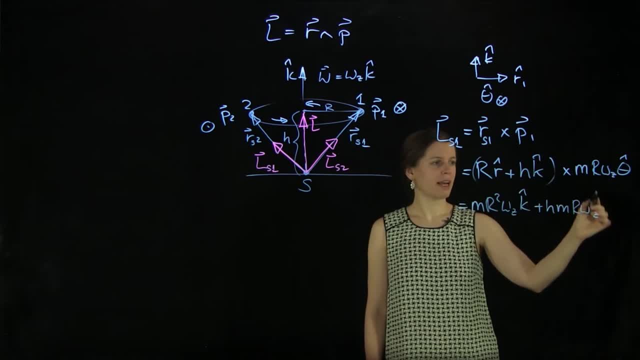 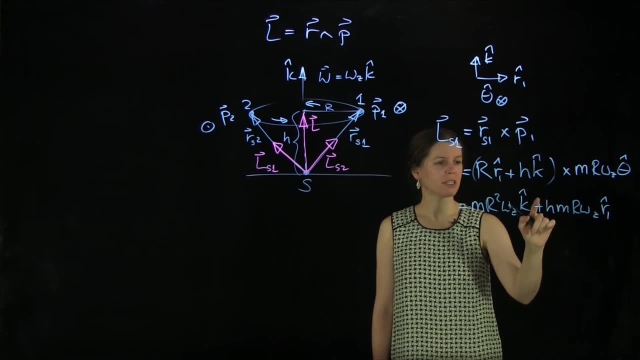 And then we have k hat, cross theta hat. That's anti-cyclic. And we get an r hat, And this is, by the way, an r1.. And this is an r1. And we get a minus because it's anti-cyclic. 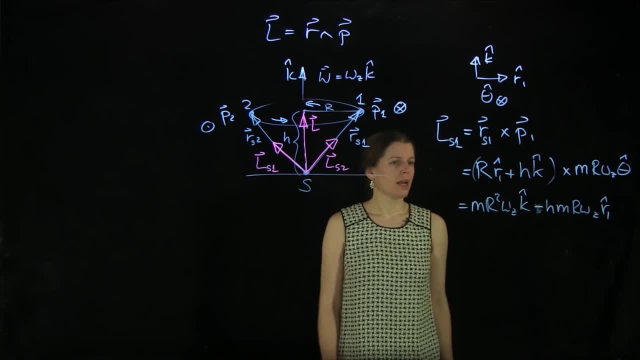 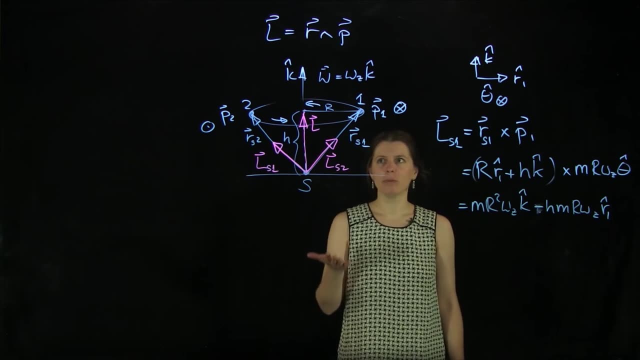 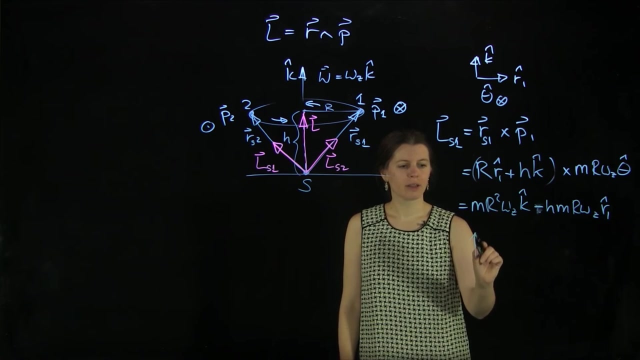 So we're going to turn this here into a minus, And that is the angular momentum for our first particle. Now we're going to do the same in an analogous way for our particle number 2.. But again we need to look at the coordinate system. 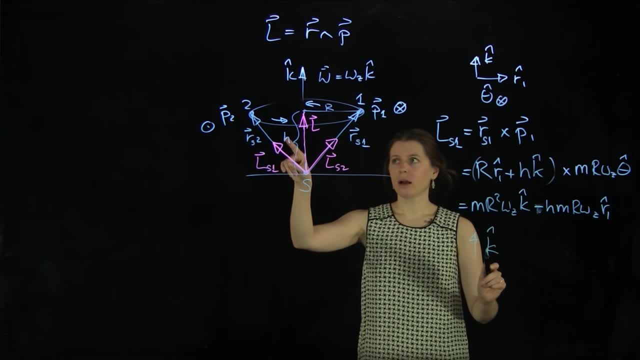 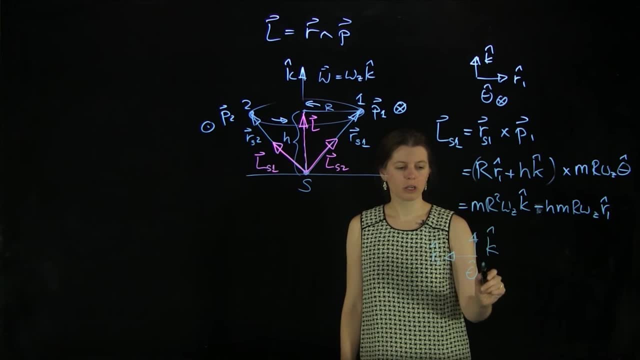 That's very crucial here. So k hat still goes up r hat now goes into the other direction and accordingly theta. So theta hat comes out of the board And then we can just write down our ls2 here as same thing.